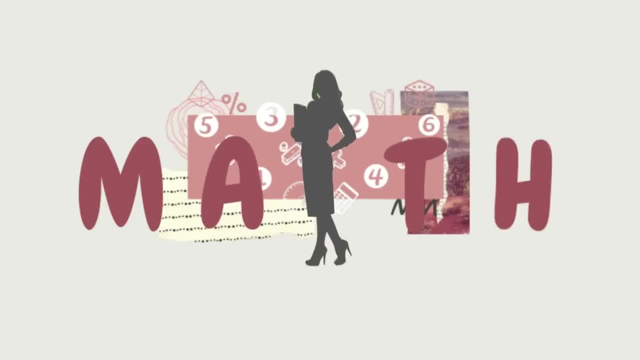 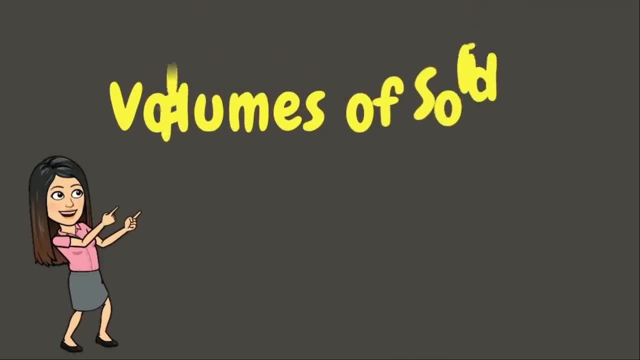 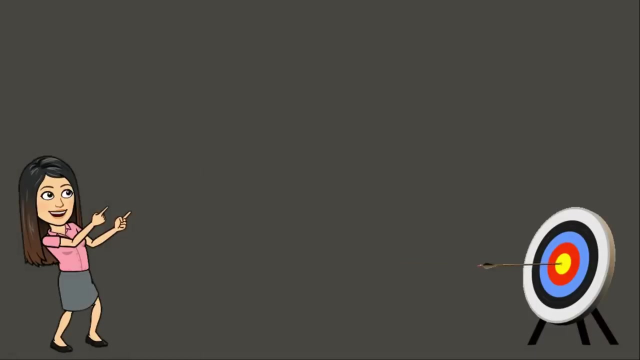 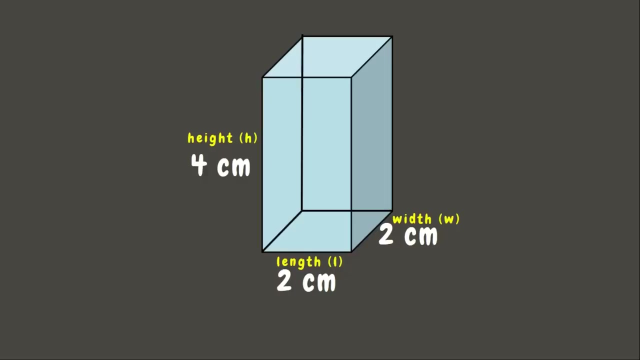 Good day students. welcome back to my classroom For today's lesson. you are going to learn how to solve 40 volume of rectangular prism, pyramid, cylinder, cone and sphere. Let's begin. We have here a tank in the form of rectangular prism. Its height measures 4 cm, length 2. 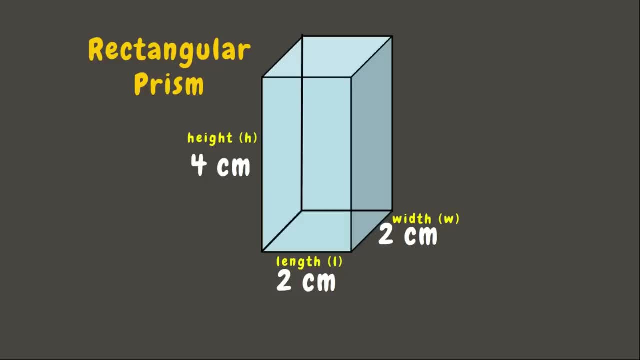 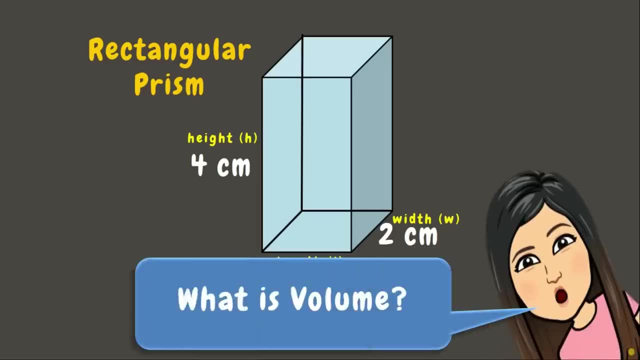 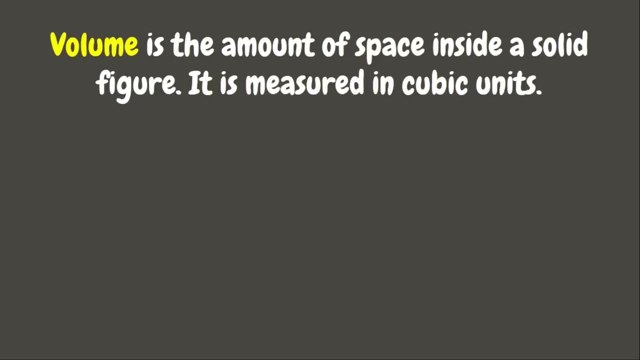 cm and width 2 cm. Now let's solve for its volume, But wait. first let's have a quick recap on what volume means. Volume is the amount of space inside a solid figure or three-dimensional figures, unlike the area, which is measured in square units, and volume, it is measured in cubic units. 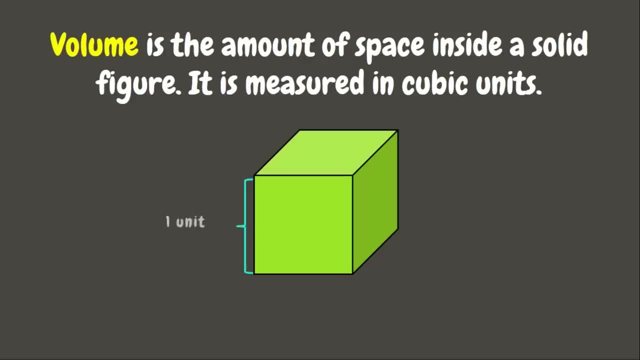 Cubic unit is a cube whose sides measure 1 unit. If each side measures 1 cm, the volume will be 1 cubic chamber. If they're 1 meter, it will be 1 cubic meter. Now if we have two cubes whose sides measure 1 centimetre, then the volume of those sides 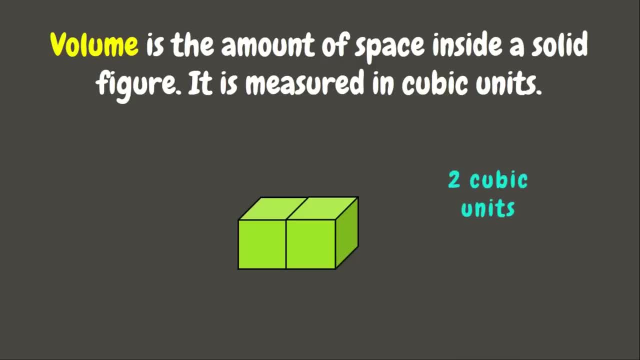 1 unit, the volume would be 2 cubic units. If we add 1, that will be 3 cubic units. And let's say we have 3 more, that will be 6 cubic units. Here we can see that we have formed. 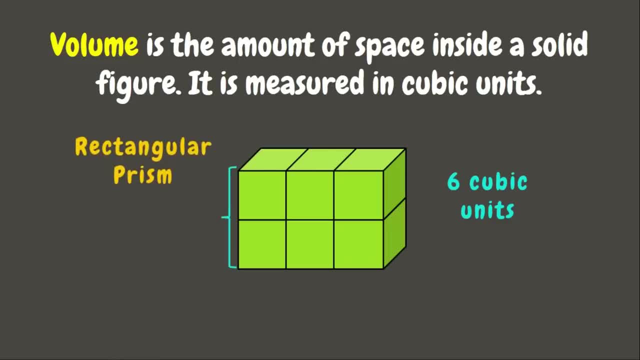 a rectangular prism whose height measures 2 units, length 3 units and width 1 unit. We can determine the volume of a figure by counting the number of cubic units that can fit inside it. Now let's try and go back to our problem. 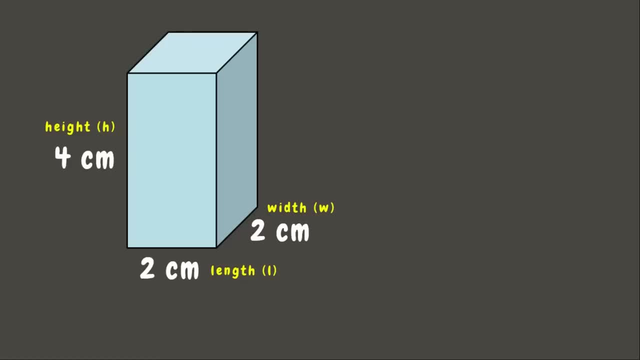 Now let's try to make some cubic units using the dimension of this figure. Here the rectangular prism has the height of 4 centimeters. It means that it has 4, 1 centimeter, so that will be 1., 2,, 3, and 4.. For its length it has 2 centimeters, so that will be 1, 2.. And for its width, it: 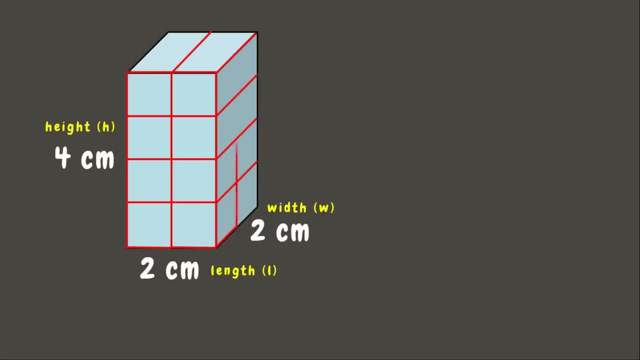 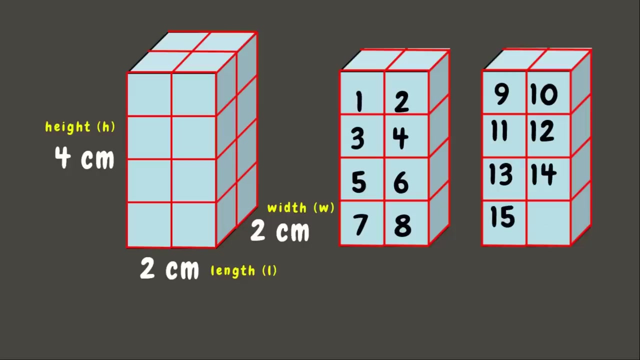 has 2 centimeters as well, so that will be 1, and 2.. Now we can see that we have formed some cubic units. Now let's count them. Now we have 16 cubic centimeters, and that's the volume of this prism. Now we can observe. 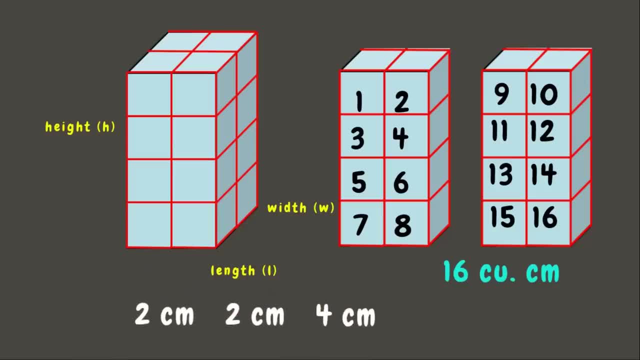 that if we multiply 2 centimeters to 2 centimeters to 4 centimeters, we will get 16 cubic centimeters. This means that to get the volume of a prism we can simply multiply the length with end height, So that will be length w- h. Also, we can observe that the length times width is the 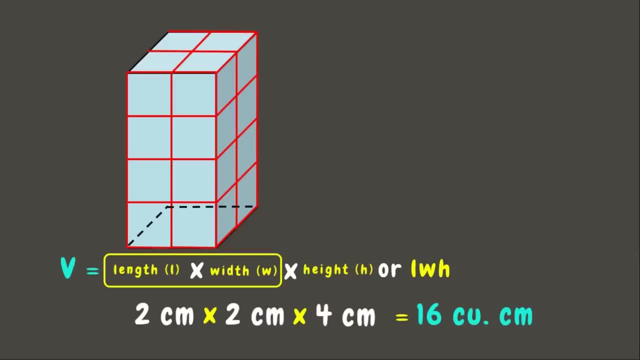 area of the base. Therefore, we can also say that to get its volume we can multiply the area of the base times the height, So that will be b times height. Now, as we can see, we are also multiplying 3 dimensions. 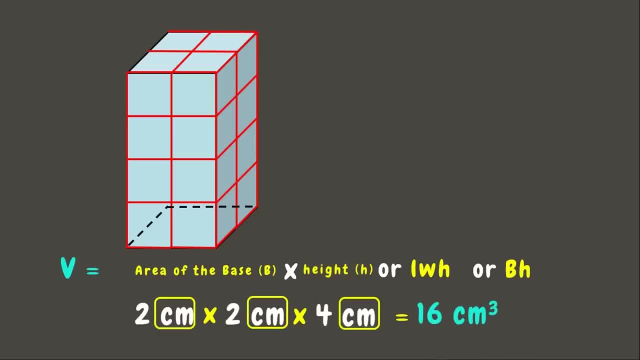 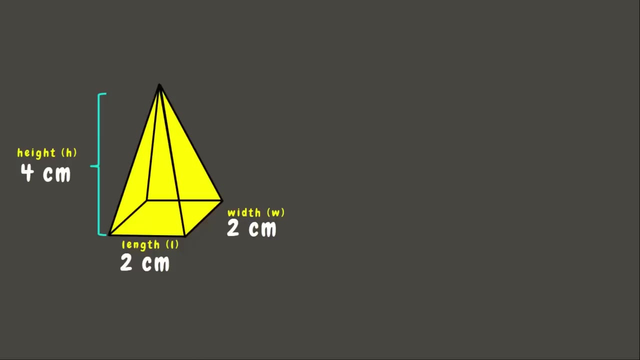 Therefore, we can also write the answer as 16 cubic centimeters, with 3 as the exponent: Wonderful. Now let's have another example. Next up, we have pyramid whose height measures 4 centimeters, length, 2 centimeters and width. 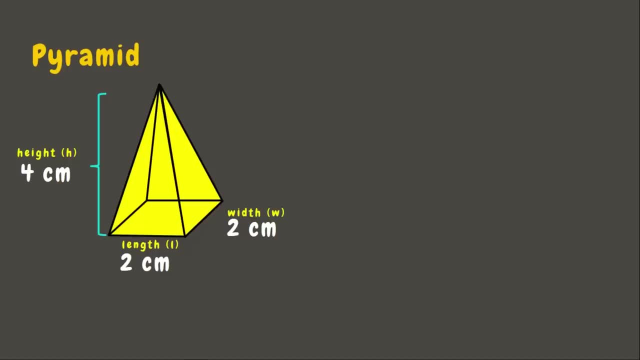 2 centimeters. In our previous video lesson we learned that 1 rectangular prism is equal to three pyramids, considering that they have the same height and base. Therefore, we can say that the volume of a pyramid is one-third of the volume of the rectangular prism. So the formula for the 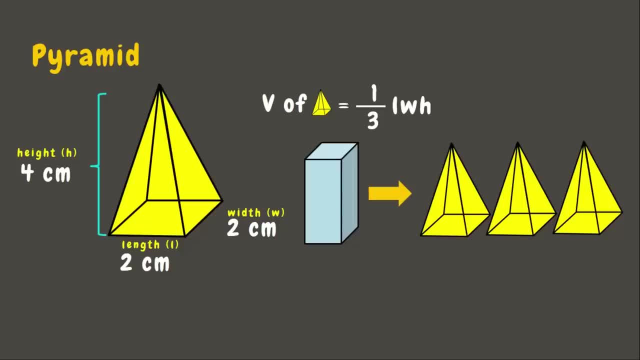 pyramid's volume is one-third length times width times height, or length times width times height, divided by three. Now let us solve The length here, which is two centimeters times the width, which is two centimeters times the height, which is four centimeters divided by three: Two times two. 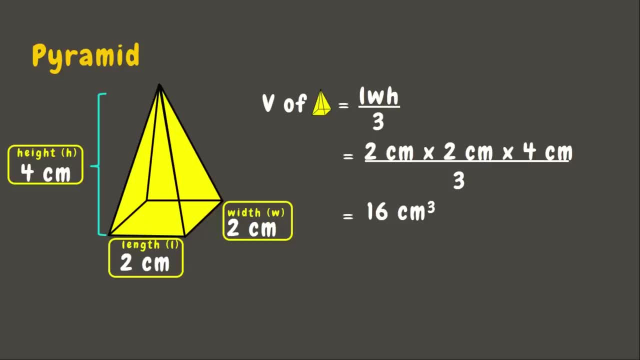 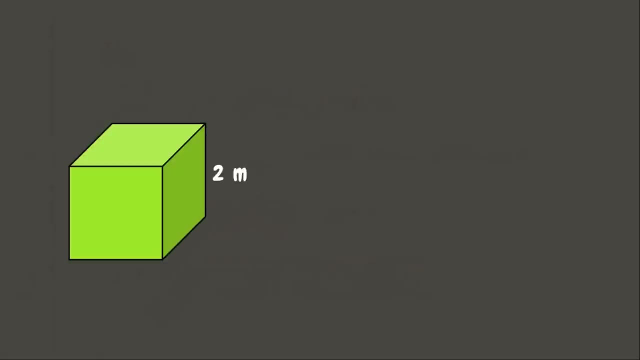 times four is 16 cubic centimeters. divided by three, That is 5.33 cubic centimeters And that's the volume of this pyramid. Great job. This time we have a cube whose sides measure two meters. To solve for its volume, we need to. 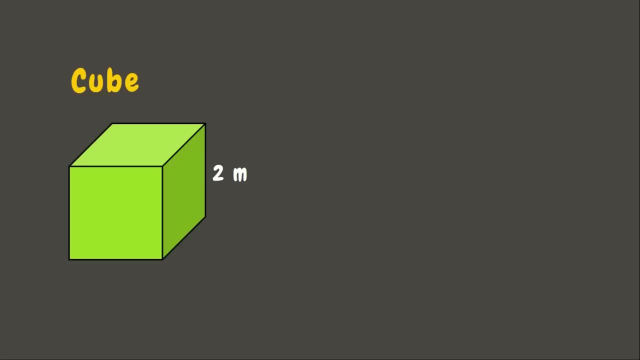 multiply the length to its width, to its height. But since the cube has equal sides, we can have the formula as side times, side times side or s cubed. So that will be two meters times two meters times two meters, Which is eight cubic meters, And that's the volume of this cube. 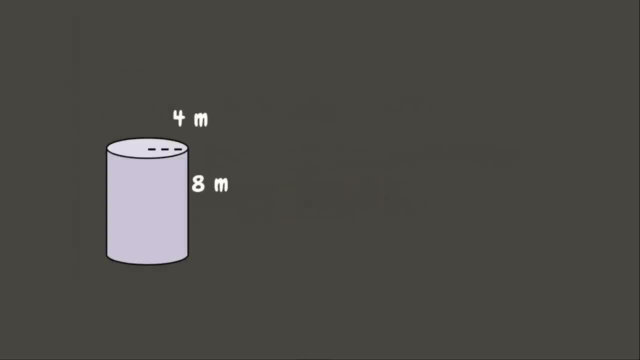 Great job. Step 4: fruit. Now let's have another example. This time we have a cylinder whose radius measures 4 meters and the height is 8 meters. The formula for the cylinder's volume is pi r-squared h. Now let us solve. 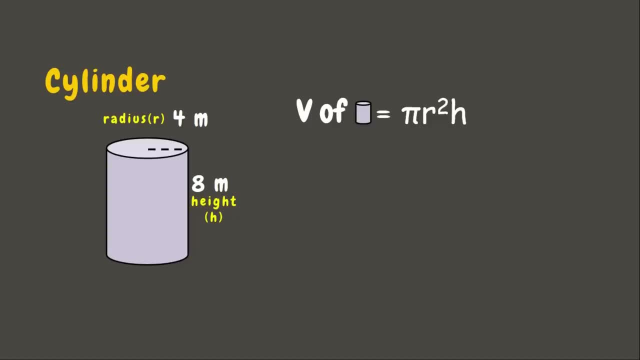 The volume of the part that we are going to use is pi r squared h. The roman formula for the volume is 7.25. pi r squared h to use is 3.14, so that will be 3.14 times the square of the radius, which is 4 meters, so that 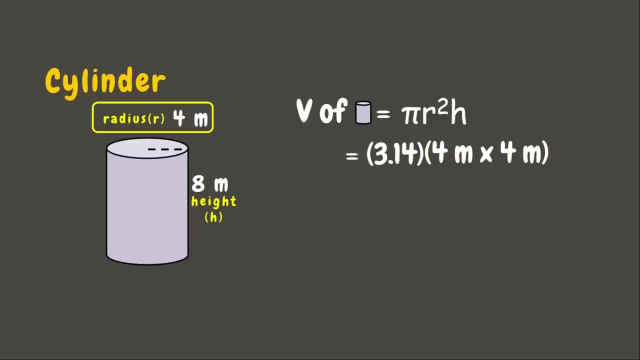 will be 4 meters times 4 meters times the height, which is 8 meters. first, let's simplify: 4 meters times 4 meters. there you go. now we have 3.14 times 16 square meters times 8 meters, 3.14 times 16. 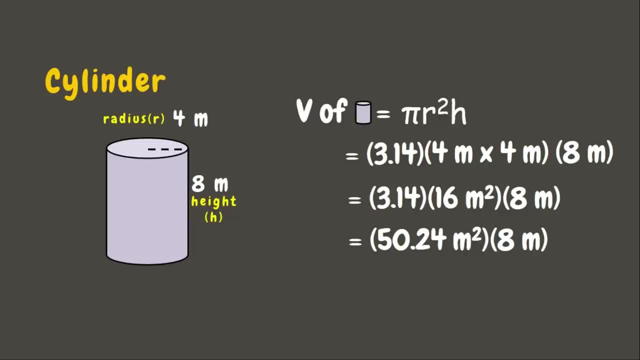 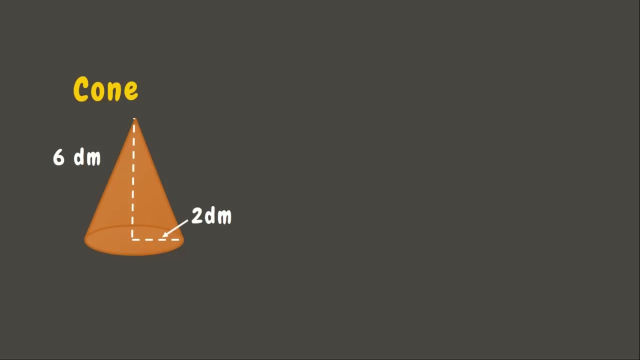 square meters is 50.24 square meters, and if we multiply that to 8 meters, the answer would be 401.92 cubic meters, and that's the volume of this cylinder. awesome, now let's go to our next example. next up, we have here a cone whose height measures 6 decimeters. 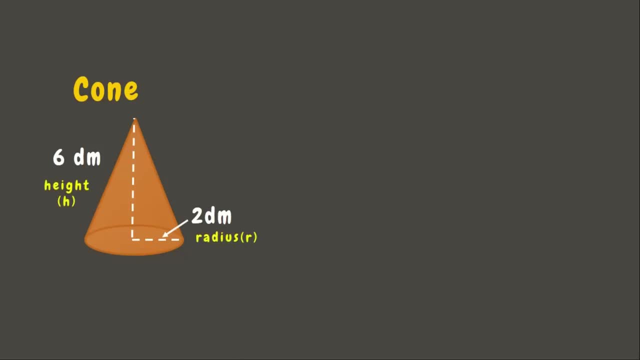 and the radius is 2 decimeters. from the previous video we learned that one cylinder is equal to three cones, considering that they have the same height in base. therefore, we can say that the volume of a cone is one-third of the volume of the cylinder. so the formula 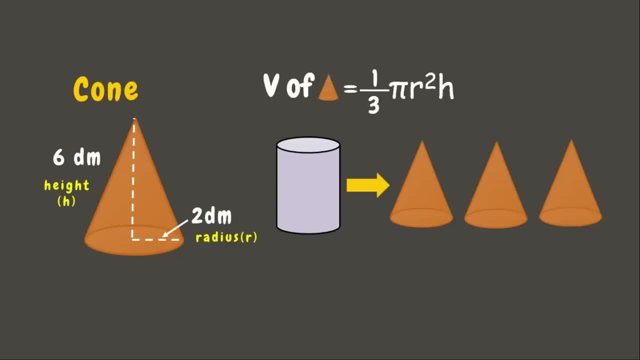 for the cone's volume is one-third pi r squared h or pi r squared h divided by three. now let us solve the value of the pi, which is 3.14 times the square of the radius, which is 2 decimeters times 2 decimeters times the value of the height, which is 6 decimeters divided by 3. 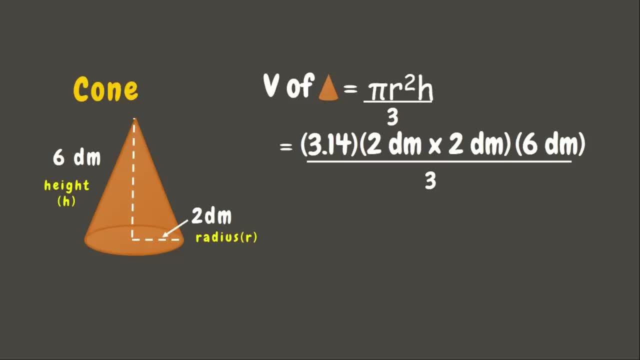 first, let's simplify: 2 decimeters times 2 decimeters, which is 4 square decimeters. next, 3.14 times 4 square decimeters times 6 decimeter is 75.36 cubic decimeters, and if we divide it by 3, the answer would be 25.12 cubic decimeters, and that's the volume of this cone. 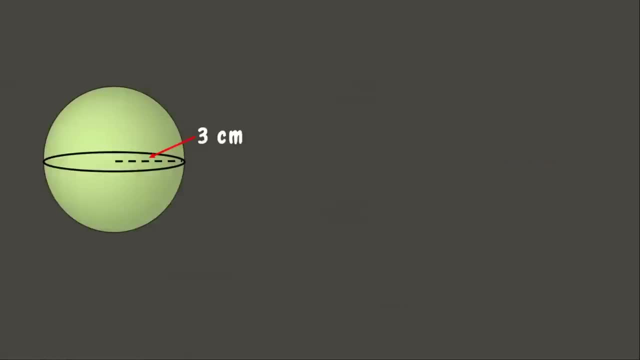 great job. for our next example, we have a sphere whose radius measures three centimeters. the formula for the volume of the sphere is four-third pi r cube, or four times pi r cube divided by 3.. now let us solve four times the value of the pi, which is three point fourteen. 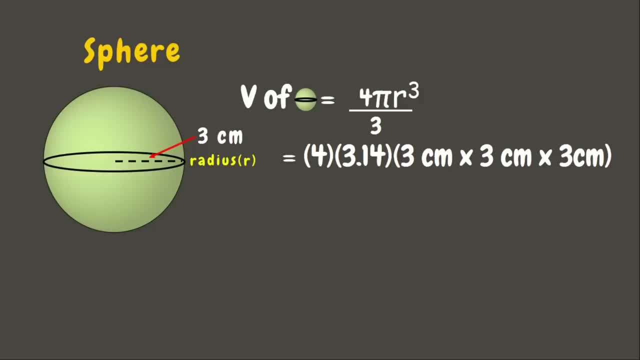 times the Q of the radius, which is three centimeters. So that will be 3 centimeters times 3 centimeters times 3 centimeters divided by 3.. Now let us simplify. first, We have 4 times 3.14 times 27 cubic centimeters, divided by 3..